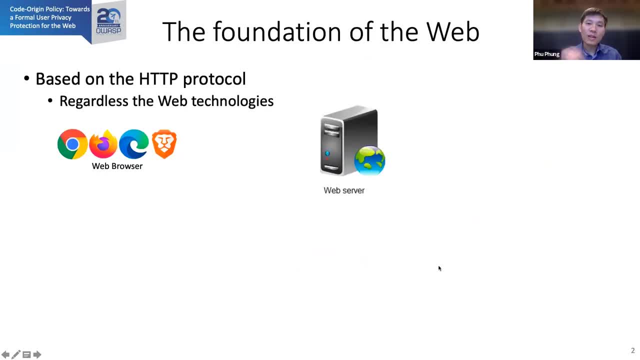 right, So let's review about the foundation of the web a little bit. I assume that everyone is familiar with the web, But the business is pretty smart. I mean, we are still on the same page in this. So the web even like. how many evolution. 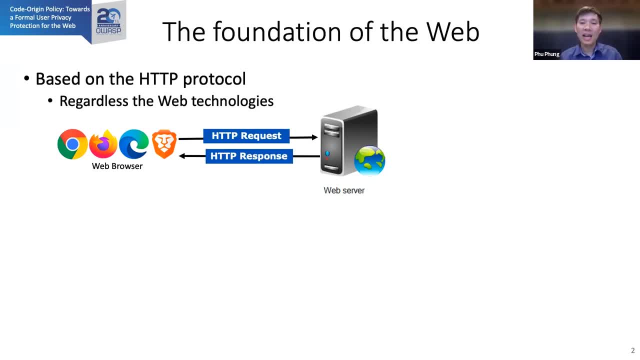 or something happens in the future. The web technology right now is still based on the HTTP, And nowadays the web contains a lot of other things, But the thing that is the basic of the web is they have just the plain text with HTML, JavaScript. 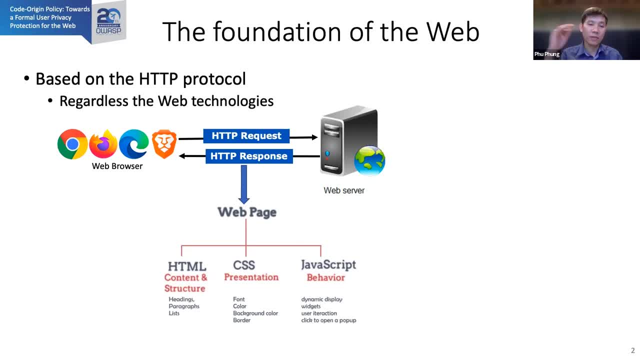 and also some CSS for the execution in the browser. So nowadays, if you can see from the picture earlier, web 3.0 have a lot of code running in the browser. It's kind of the edge computing And here in statistics you may know. 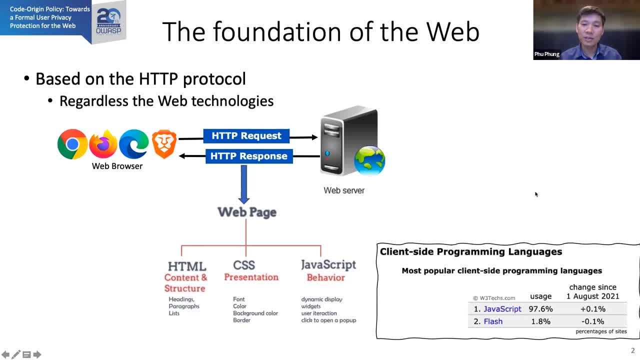 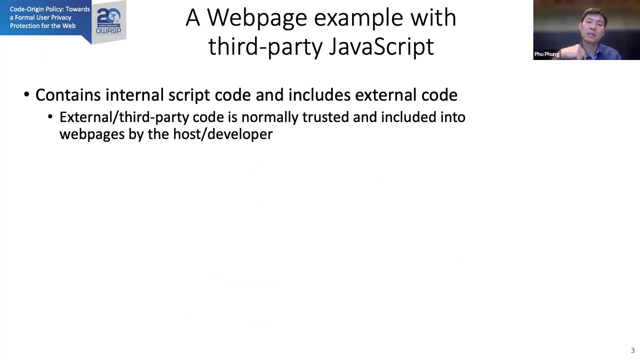 that JavaScript is now in every single web page, right? And that is the dominant programming language for the web, right? So let me give you some example. Let's talk about the typical web page or website web application nowadays. So normally it's not only just what you see. 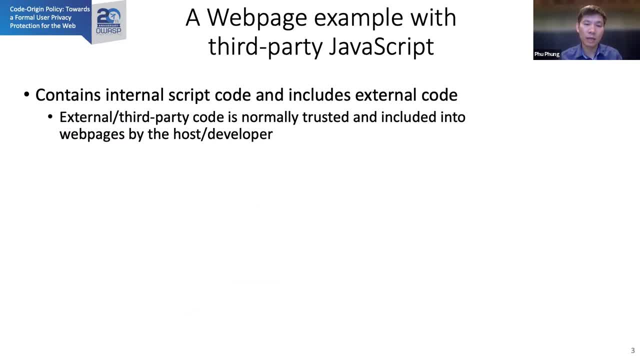 It also has a lot of internal and external code running behind the scenes right, And normally it also includes the third-party code And when, for example, you're working on a web page or your website, include the code from somewhere else. normally you trust that code. 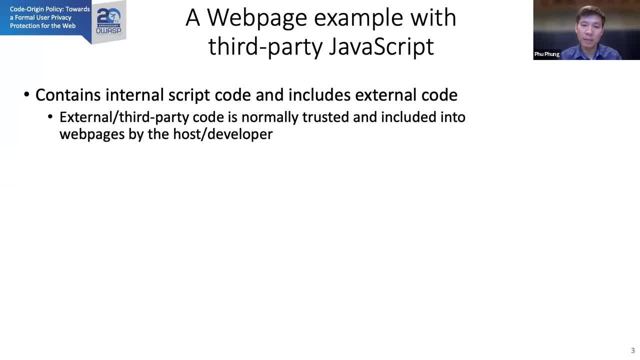 And you include that, The developer will include that. I mean here I call that by the host or the developer. So here I just show you an example that we see on the left-hand side, we see at the user, But on the right-hand side you see there. 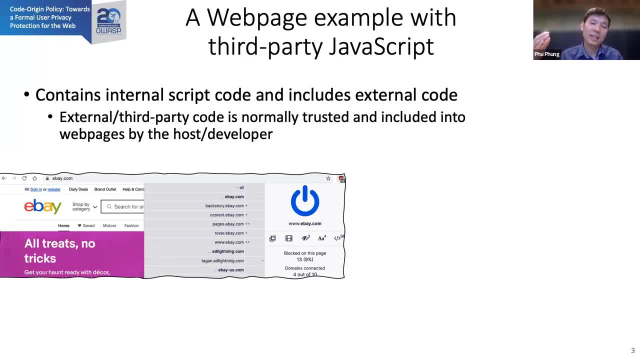 is the tool that I use in my browser. They display for like how many Like external domain and the code that's included by you know, in this case ebaycom, And there are also other tools that they know that they track. 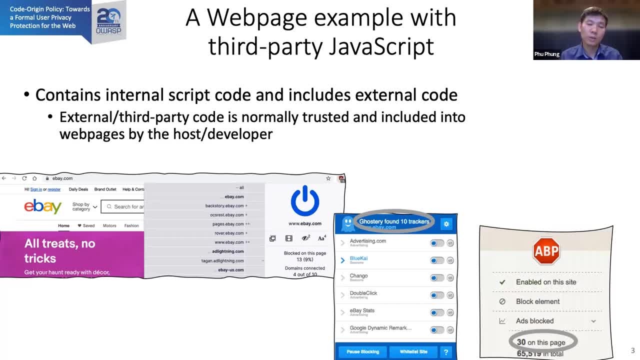 They know like how many trackers that track you during this visiting to the web, right, And these are. by the way, these are popular browser tools like uBlock, Autogencom or WhatsAppcom. I don't know if you guys are familiar with that. 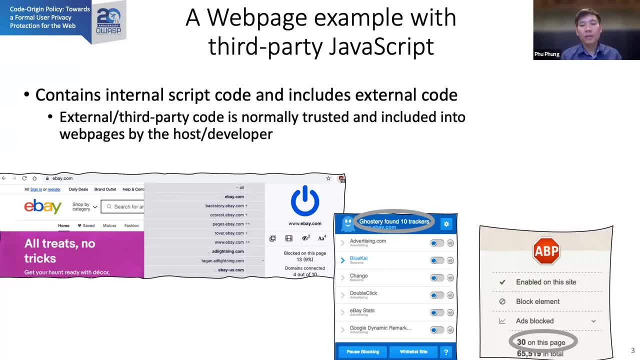 But you can use it to track, you know, like what's three or ad block, something like that, right? So this is the general web application and the web in browser right now. So my research is about like security and like you know. 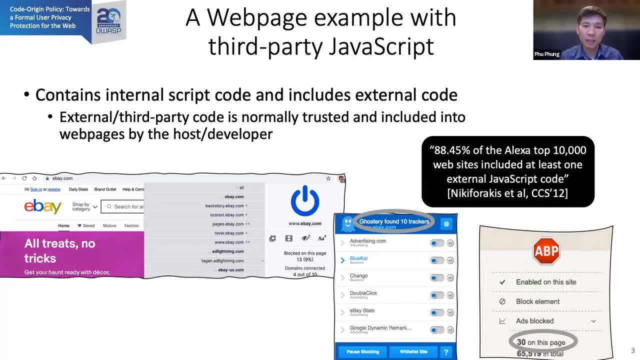 the concern and the privacy concern about the web right now for the user. So let's review about the oh. by the way, there are like a lot like most of the top 10,000 websites include like external web. 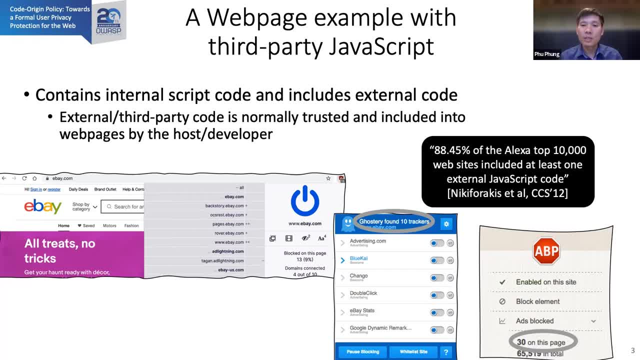 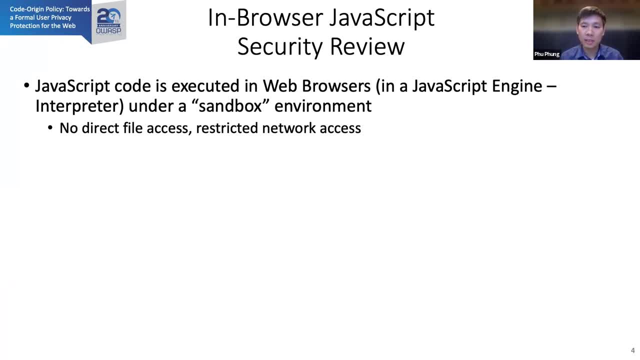 That is a typical one that I just want to say, right. So I want to review about some major security mechanisms in the browser for JavaScript code. that, because it's run in the browser, So JavaScript code download from the remote server normally And then it's run inside the browser right on the fly. 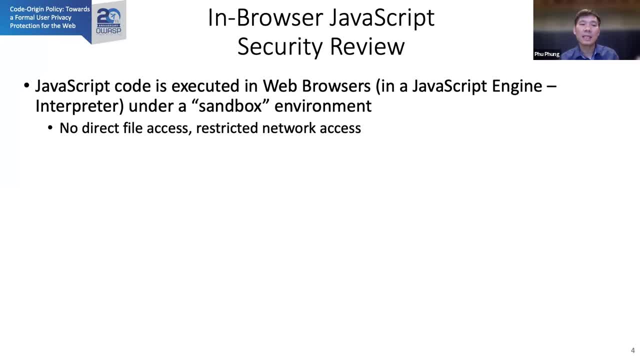 So the security of course must be guaranteed And in this case the execution will be in the sandbox environment. Of course the code cannot direct access to your computer And they have some limitation about the access to computer. Otherwise they can do whatever they want in the computer. 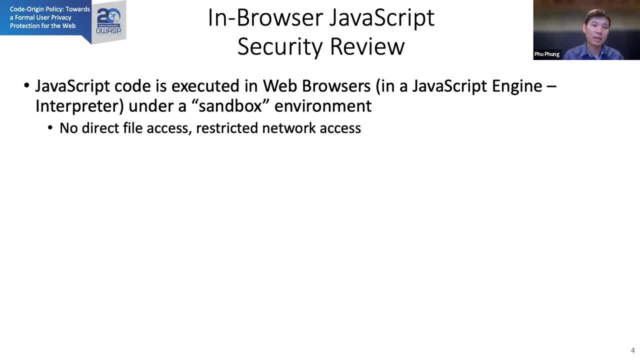 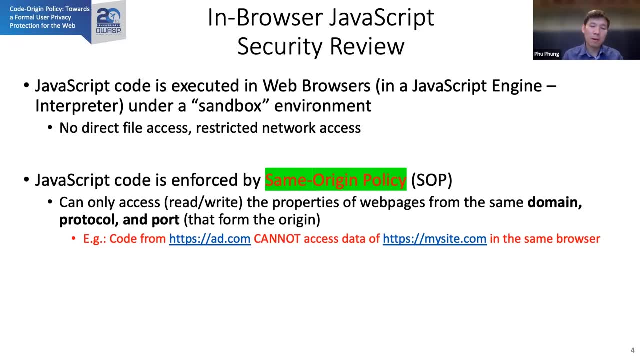 right, That is one mechanism. The other mechanism, And it's well-known in the web, It's called same origin policy, right? So assume that because the browser opened like too many websites at the same time and the user can visit different site. 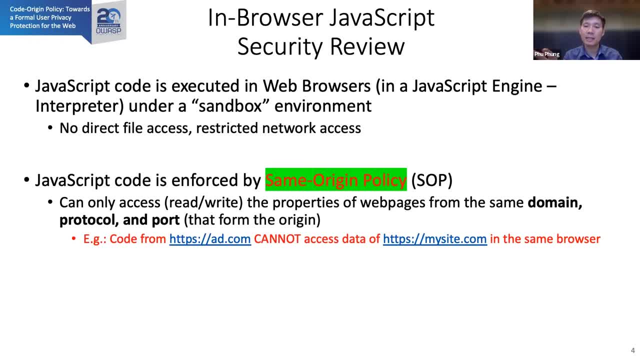 So there are some confidentiality inside that site And then the browser only keep for that website. So, for example, you may know about cookie right. So cookie, the sensitive information, And it's only, It's only shared among the origin. 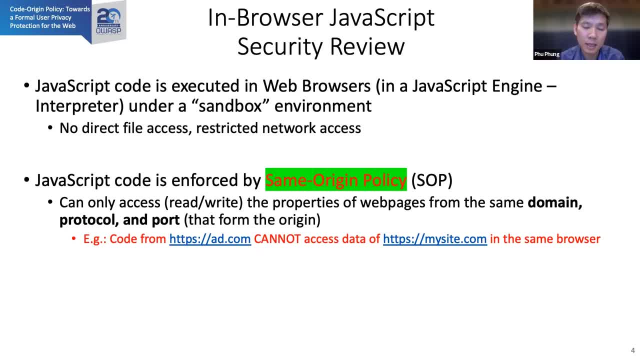 Origin is stand for. it's formed by domain protocol and the port right. So example here: if you include, if you are in this domain, you cannot access the data of the other domain right. So that is one major security mechanism. 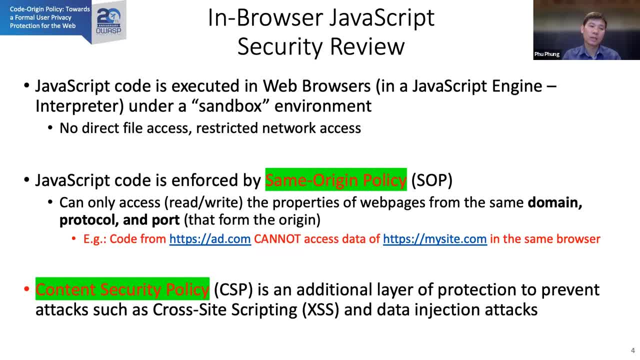 And the other one- One later on- was called content security policy. It's this additional layer to protect the attack. For example, one of the most popular attack is cross-site scripting attack, that the attacker can inject JavaScript code and execute JavaScript code right. 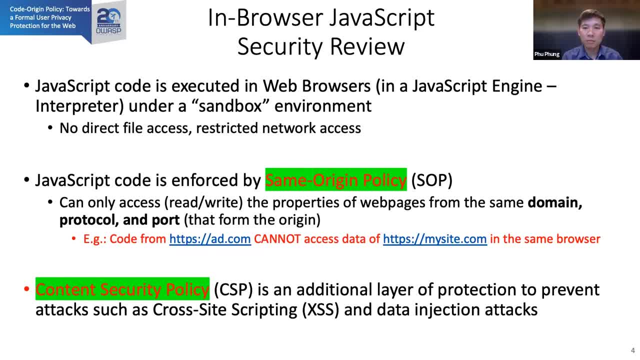 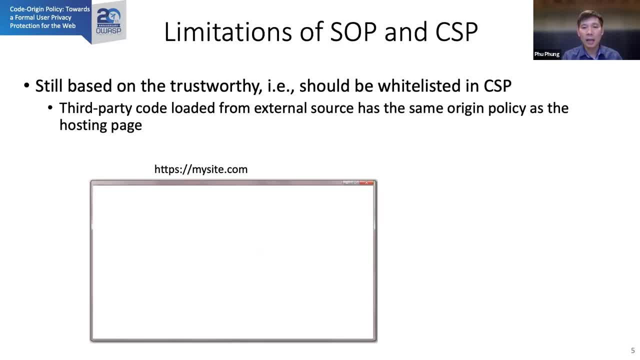 However, there are some limitations with this mechanism, right. However, there are some limitations with this mechanism, right? So let I give you a scenario where, let's say, the website, like, for example, mysitecom, includes the code from: 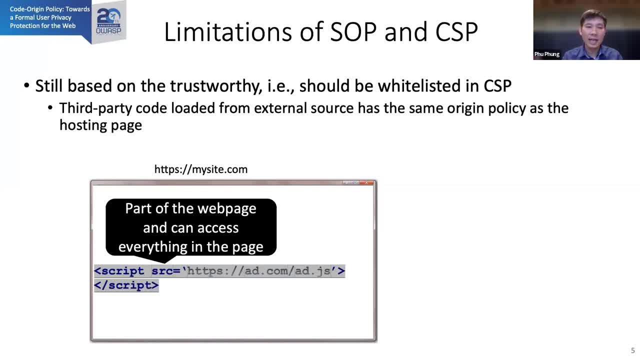 let's say adcom, as I mentioned. So in this case, you see that when we include the code from external domain or remote domain right, this code is a different domain Right. However, when it's in blue, it belongs to the same origin. 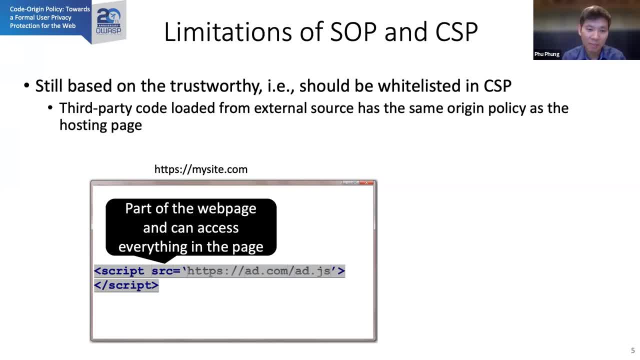 as the hosting page, Like in this case, it will be mysitecom right. So the issue here is that- and this is still the limitation for this- is that when mysitecom includes the code from adcom, the mysitecom developer. 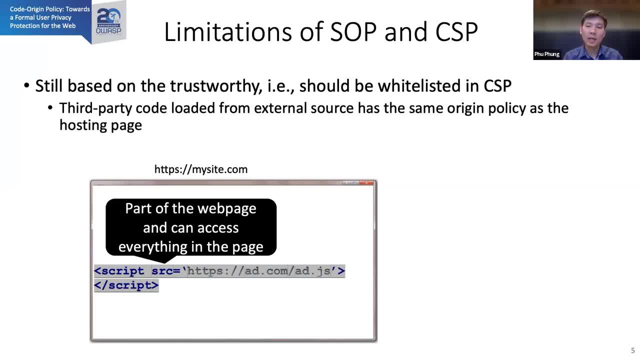 or I mean in this case the account provider always trusts that adcom will not ham or will not do maliciously in that mysitecom of course right. So this means that it's beyond the trustworthy right. So the provider will trust its partners. 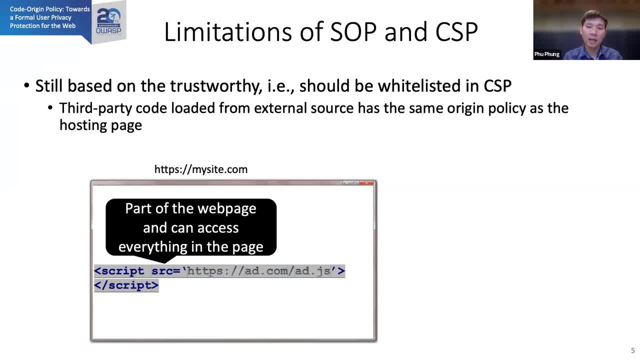 that the code will be included, And then, of course, in that case the provider has to wireless this third party saying that, OK, you are allowed to do this. But the issue here is that in the scenario, the code is not controlled by mysitecom. 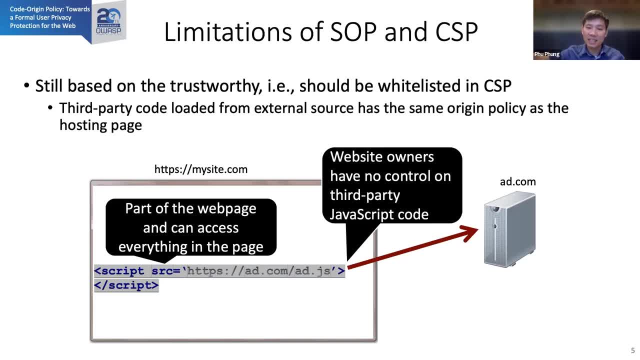 in this scenario, right, So it's hosted outside. It's hosted outside, And then I mean, in reality, the code can be chained at any time. right And seriously. there's a case that the code hosted by outside can be compromised by attacker, not mysitecom. 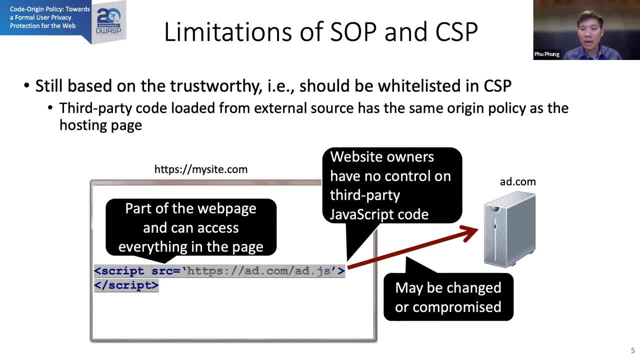 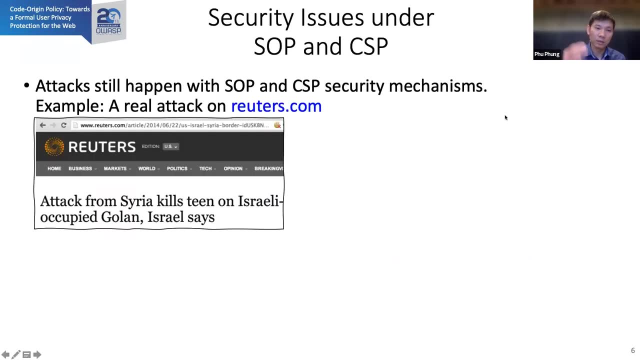 but adcom, for example, right. So in reality that kind of attack like happened, right. So let me give you a real example that happened years ago, Like on the website you may know about. It's rogercom, right. 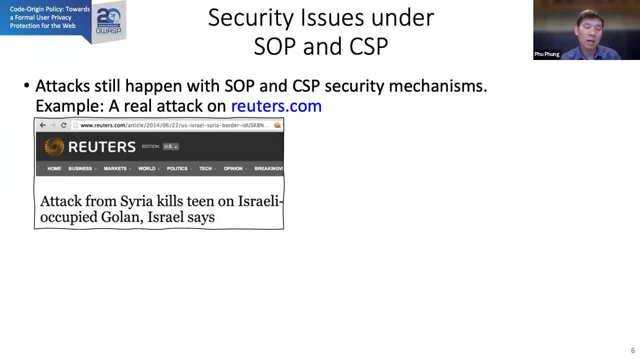 So a couple of years back a user of the rogercom experience that when they visit an article news it's redirected the usercom It's redirected to an attacker page like this And it's happened in the past. So the common sense in this scenario. 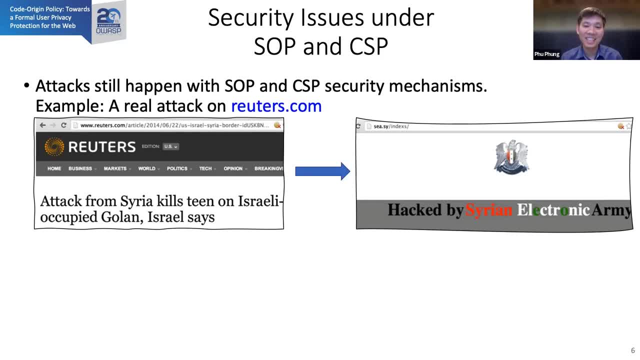 clearly that rogercom server will attack, right? I mean that is the user of the roger. OK, Something wrong happened on rogercom, right? But actually it's not like that. Actually, rogercom has not been attacked. 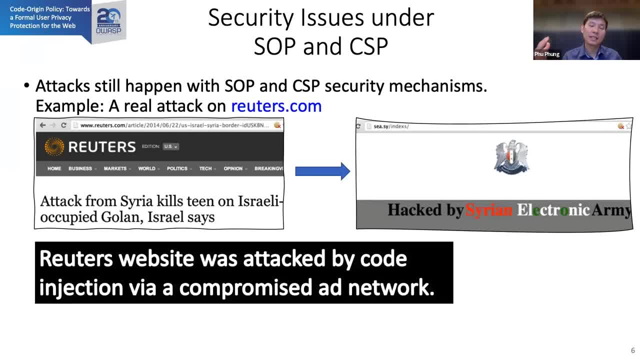 But rogercom On the website. it's attacked in this scenario by a code injection via the compromised ad network. So the attacker injects the code in the advertisement network And in this case you see the scenario I showed earlier. 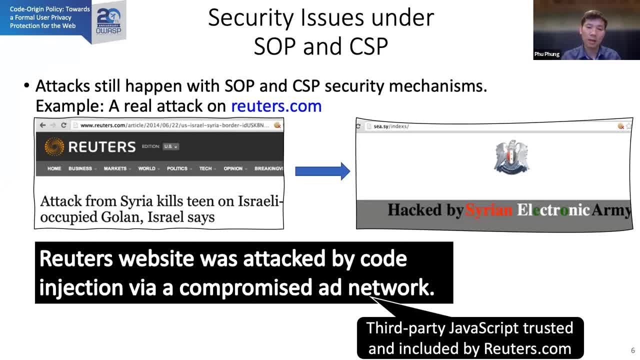 right. This is a kind of third-party JavaScript And normally when we include like that, it's thirded by the rogercom in this case, Because this is very common. You know The revenue system right. So at the user. what do we concern about right? 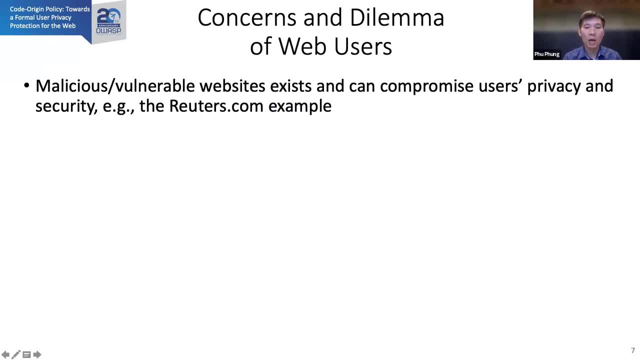 At the user. So in this case, for example, what are we concerned about? So what do we worry about this? So rogercom example I showed you earlier is an example about security problem, But also, similarly, that is the threat of privacy as well. right, 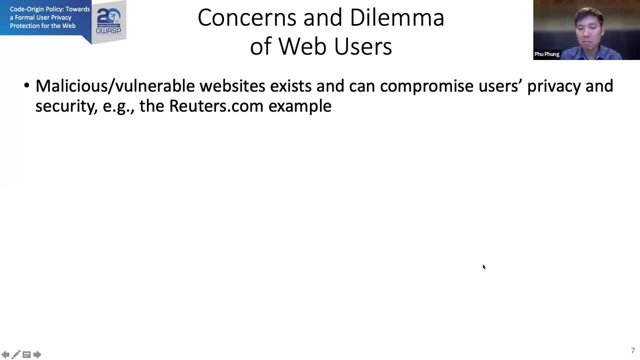 So my research is to you know, consider the like, what the user will worry about and what the user wants for this. And, most importantly, I want to protect the user from, you know, this kind of threat and also the privacy leakage. 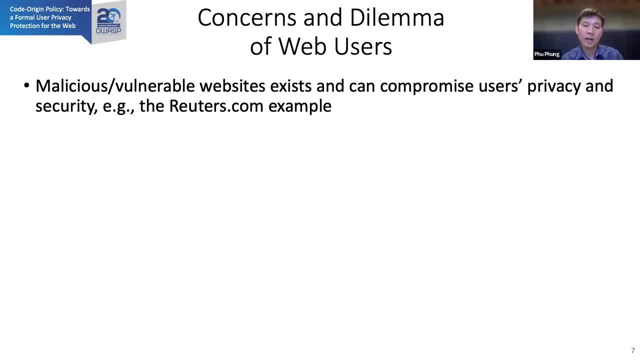 you may experience in the example of the eBaycom that I mentioned earlier, Like user having trapped right And related to this. I want to also give you a little bit of information And related to this question. there's a lot of study out there. 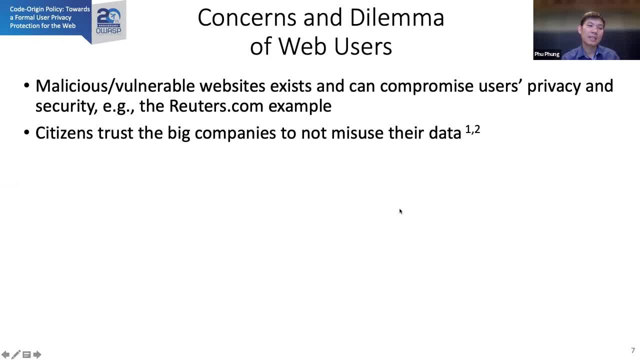 So, for example, one of the studies said that. a couple of studies said that the citizen maybe normally just trust the BITEC to take care about their privacy right, So they don't know whether the privacy will be protected or not. 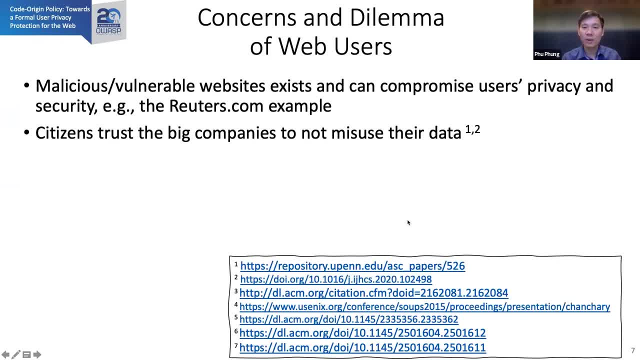 And also we also have another study said that, okay, we are not only just, for example, just block everything. They just want to receive some, you know, useful information, for example, target ads. right, They don't just block everything because that's useful to them. 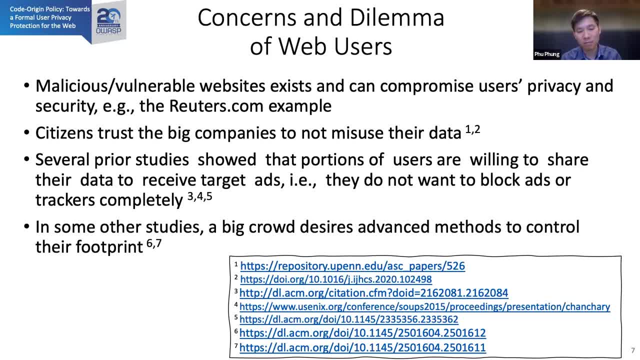 And recently there's a like design about like, where we At the user we can have advanced method to control some you know the data that can be shared. So these are the kind of, I say, the dilemma for the web user right. 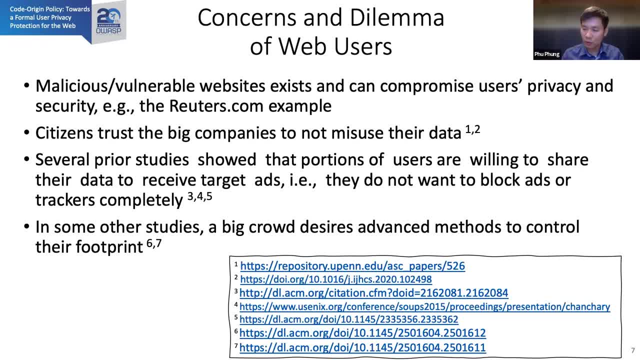 So one hand you want to have, like the protection, but the other hand there will be the- you know the way that they want to- To receive the information. For example, nowadays the AI driving in the web 3.0, right. 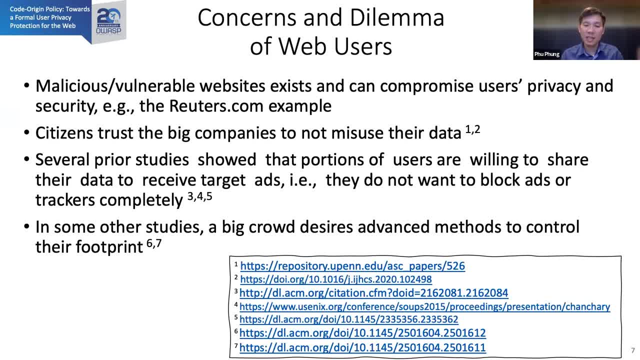 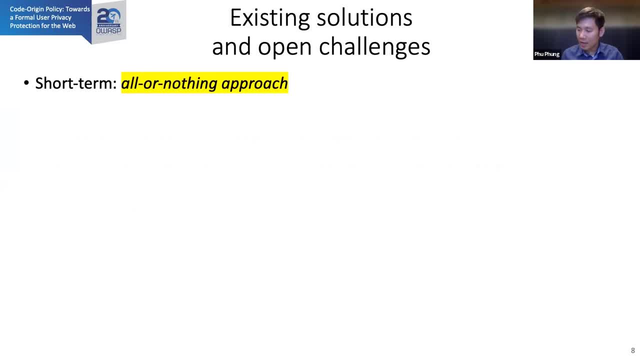 So what are the solutions currently for these types of scenarios? right, So let me review some current approaches. So, as I showed you an example in a couple of slides back, there's a short-term approach. For example, the user can install the browser extension like Blocker. 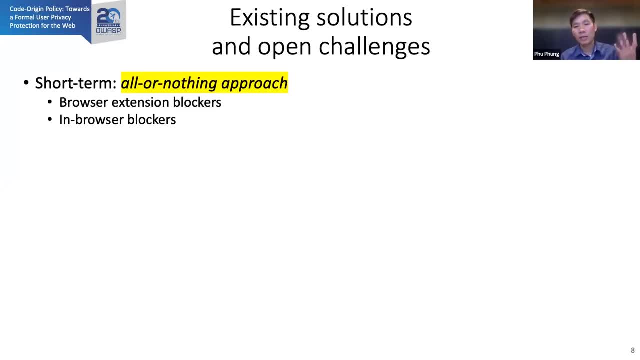 Or maybe Maybe they have an in-browser blocking, for example, Brave browser. Now they block things automatically, right? However, this has brought, as you can see, that it's still like an on or no thing, like allow or just disallow everything. 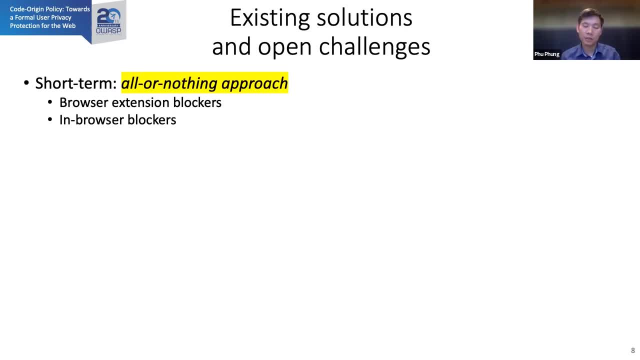 And I mean this is about the advertisement and the tracking thing and that right, So it's still not satisfied the dilemma that we just discussed right. There are also more long-term mechanisms. for example you may hear about like do not track or privacy by design or platform, like it's called P3P. 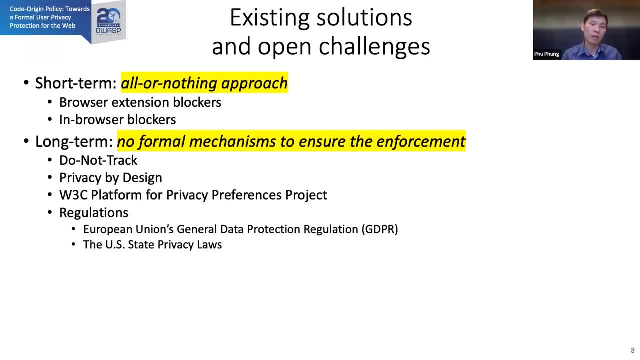 And also recently, a lot of laws- you know European law and US law- that they require the data to be, you know, tracked. So there are also more long-term mechanisms, for example, the you may hear about like do not track, or privacy by design or platform like it's called P3P. 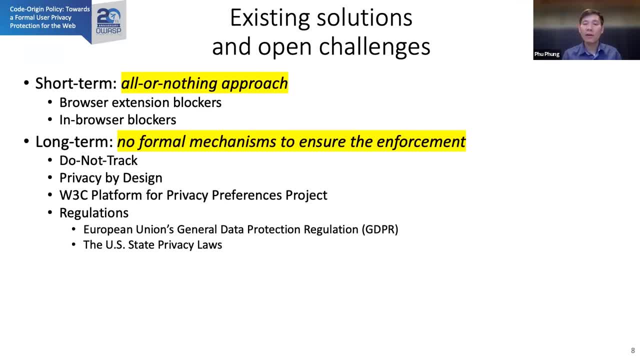 Should be protected for the user right. However, these mechanisms, it's just the- you know the mechanism, but there's no way that to ensure that the mechanism can be applied in the reality. And, additional to this, there's more open challenge for that, like, for example: 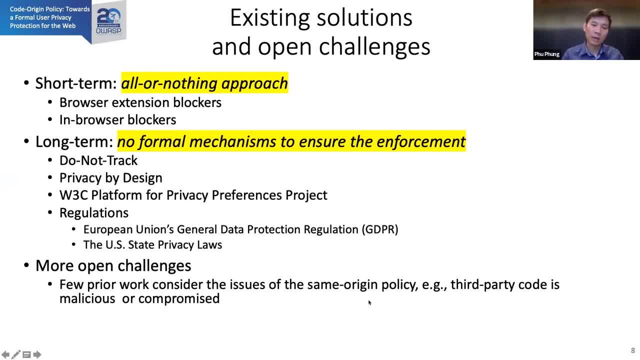 For example, I mentioned to you about the same origin policy- the third party code can be malicious or can be compromised And also there's no control from the user end to control their data to be shared or not to be shared. And, most importantly, there is no formal insurance mechanism to guarantee about if the agreement 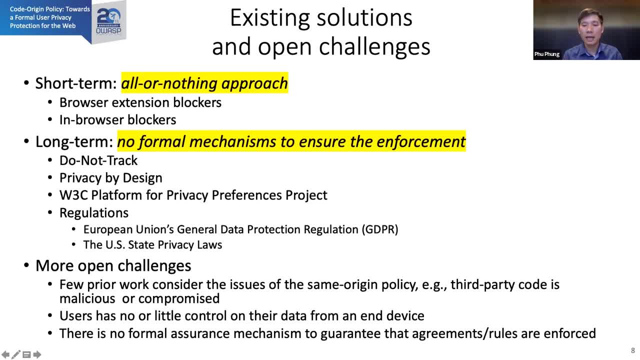 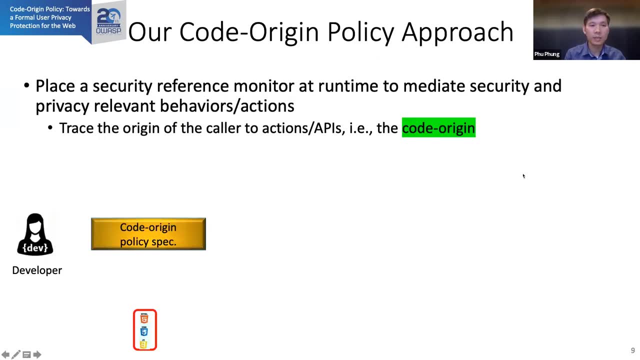 or the rule are enforced. So these are the challenges, the motivation for my work on code origin policy as broad. So I will discuss with you about the broad. So my approach is on code origin policy And the broad is to play the security reference, monitor at runtime, to mediate the security. 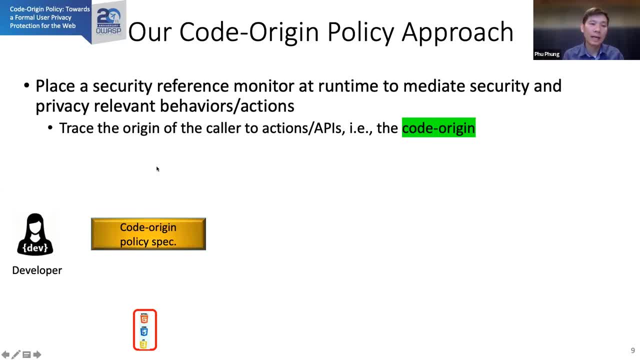 and privacy: Right, Right, Right. And the novelty here is to state the origin of the color of the API. So in that case I call it that term: code origin right. So in this approach, in my approach, the basic policy will be defined at agreement between 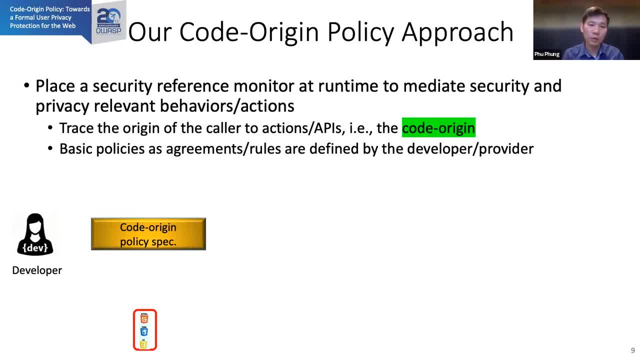 the user and the provider, And normally it will be developed by the provider and the developer. So in this feature you can see that the developer develop an app and then they can include some JavaScript code And then they can yield the code origin policy that I provide. customize that for this application. 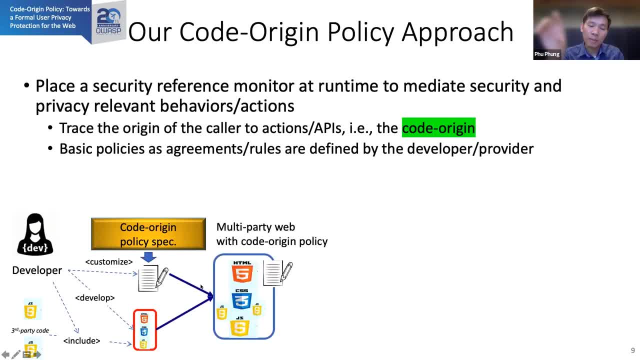 particularly, And then it's included into the pay. So in that case we have a product that we have the policy in check. The formal policy is not just agreement right And then, where At runtime, it can be enforced by a reference monitor right. 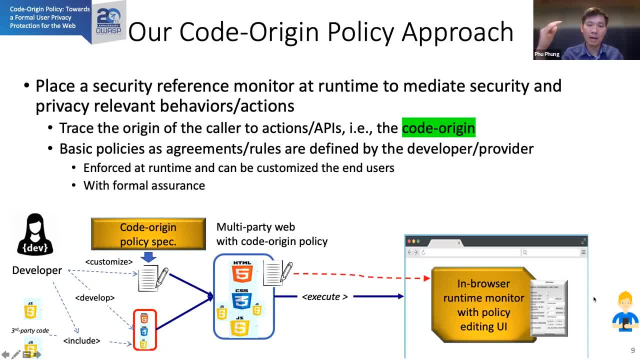 So in that case the browser can enforce that with runtime monitor And the most importantly here is that it will be guaranteed with the formal method- later on I will show you that in the other slide. But the user, in this case the user- can also edit the policy. 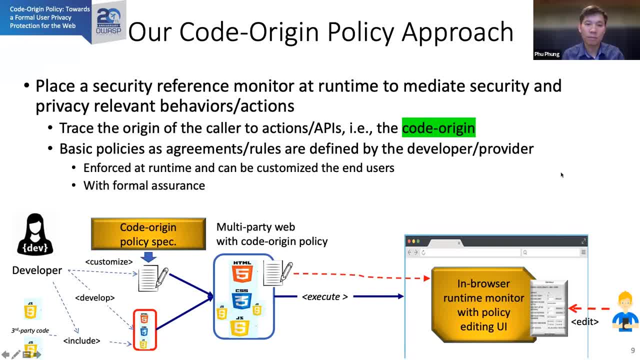 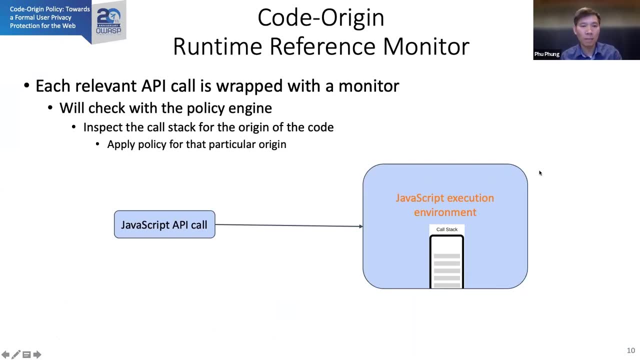 According to what they expect, right. So I give you a little bit more. it's not too deep the technical detail, but a little bit more about my approach here. So the idea is that in the regular execution the API call will be executed in the JavaScript. 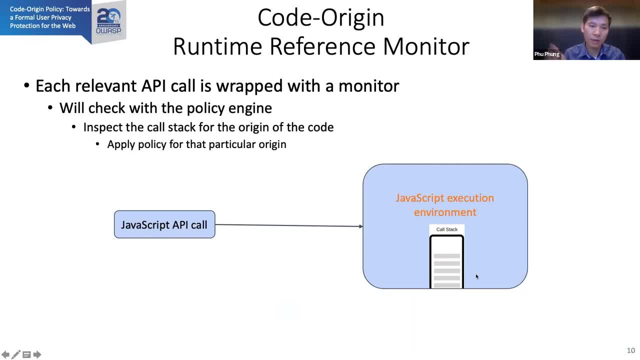 environment And of course there will be a stack to call that function, right? So our approach is that we put the reference monitor and then we disconnect this call directly. We will wrap the call to our monitor And then we have the policy and we have a code origin policy there, right? 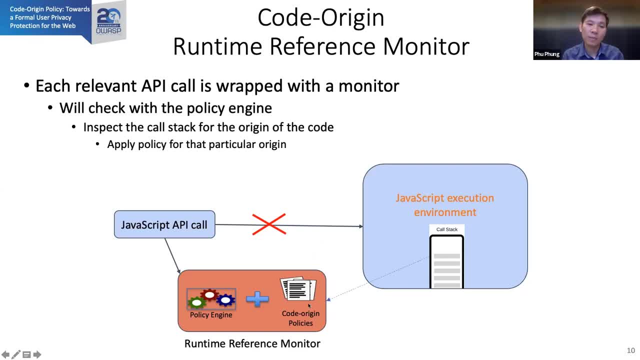 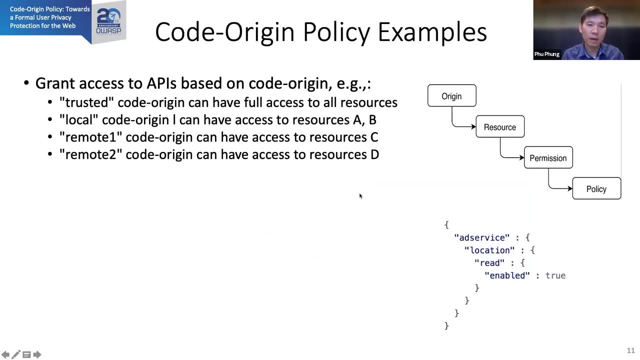 So at runtime we will also check the policy and we check the call stack to know, okay, where the code comes from, Okay, And then we execute the code accordingly, right? So I just give you some example of the code origin policy that we have. 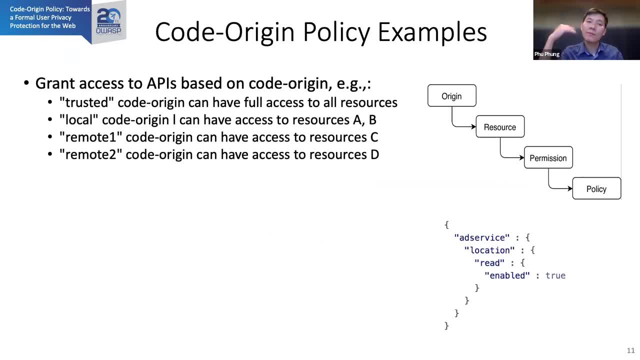 For example, we can define the policy that different origin have different access, different and different permission right. And more than that, we can have a more fine-grained policy. For example, we can define that you know, dynamic policy. 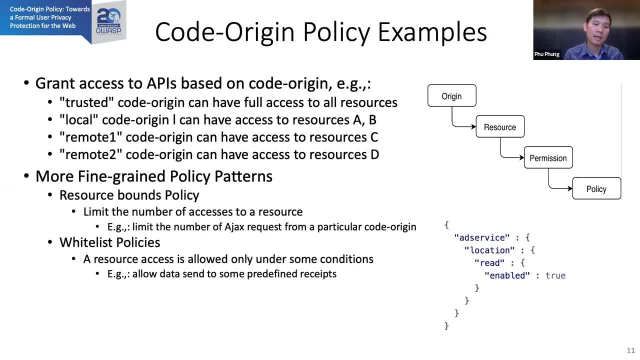 For example, the bow policy limit, the number of access, wireless policy, history-based policy, And all of these are, like, based on the code of the origin. excuse me not where the code come from right, So I give you just the illustration about one prototype implementation we did. 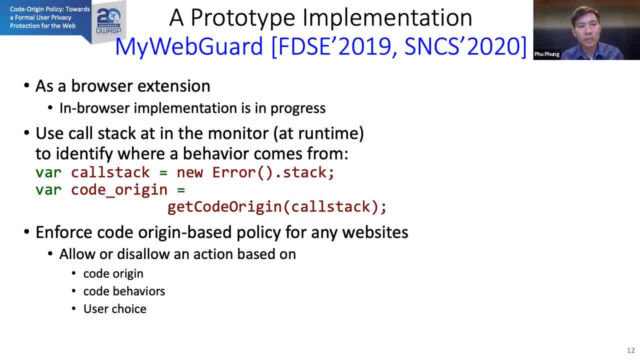 So it is. the tool is called MyWeb. We published like two years ago- Okay, So it is like two years ago- that we implement at the browser extension And during the runtime we call the stack and then we get the origin of that. 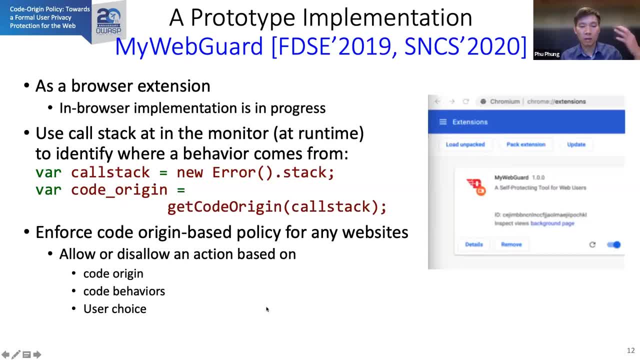 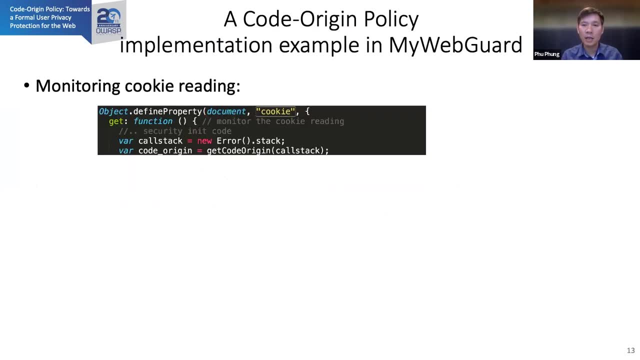 And then we apply the policy that based on the origin for the website. So a little bit more technical. I give you the example of the policy, how we enforce this. So, for example, the next policy is we monitor the code, We monitor the cookie access. 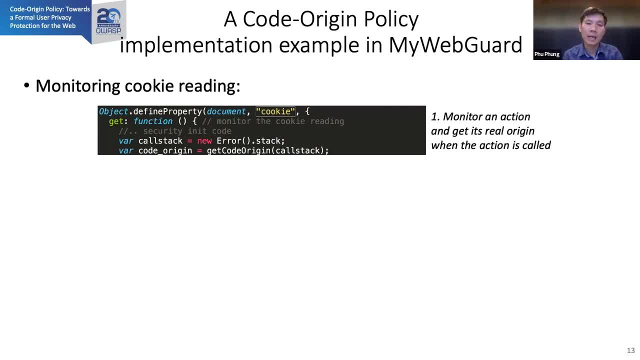 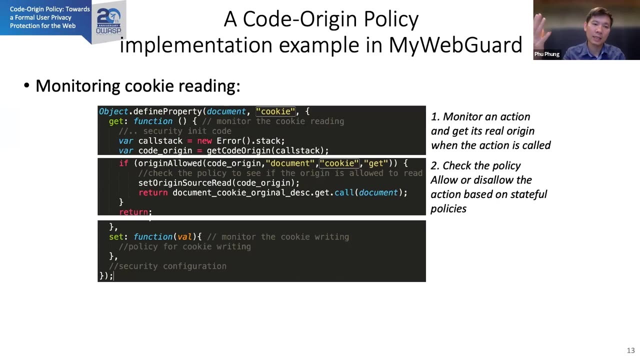 And then we so cookie access to the action, right? So we will see, okay, where the cookie, where the origin, come from, And then we will check the policy if it's allowed or not allowed, based on the idea of the code origin, where the code come from, and also the policy for that code, right? 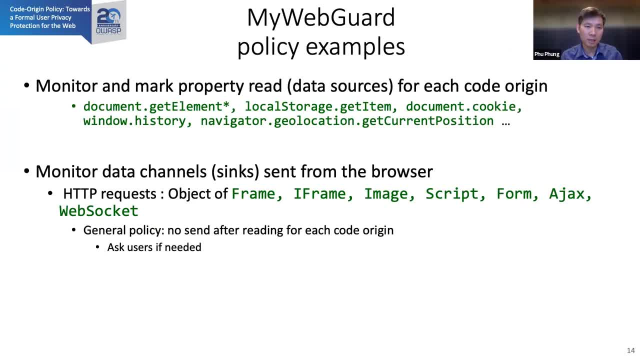 So some example we have earlier. Here is the, you know, just the basic information flow. We track the source, we, and then we track the scene. if there is the information leaked from you know shop to scene, And then we can enforce the policy, saying okay, we can do some automatically enforcement. 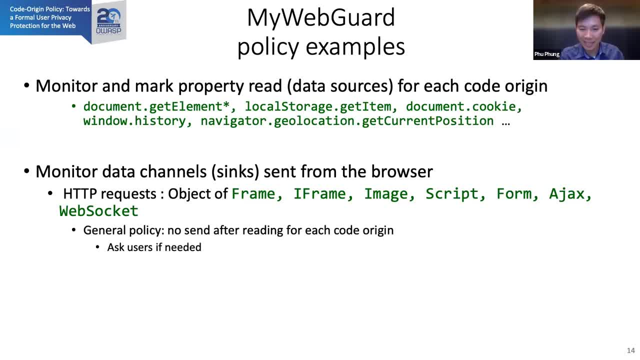 on that And we prevent something that information leaked can happen at runtime In some case. we can ask the user. Okay, Okay, So we can ask the user. Okay, Okay, So we can ask the user. okay, We can ask the user. 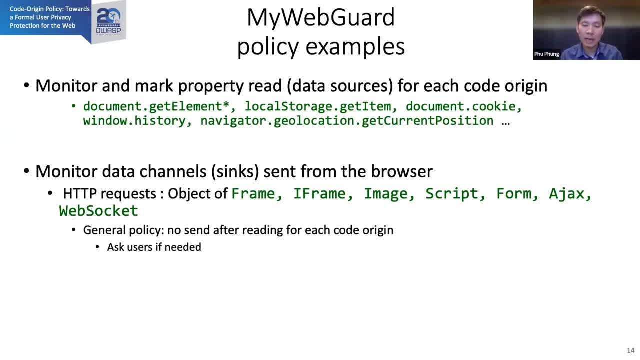 Okay, So we can ask the user. Okay, So, we can ask the user, Okay, Okay, So that's part of the code: origin policy enforcement And, as I mentioned earlier, the second part of my approach is that the formal insurance. 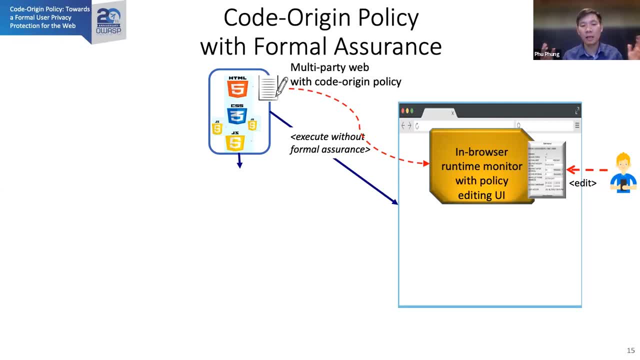 So for the formal insurance, and this is will be my long-term research vision as well. So in this vision, I anticipate that Okay mechanism will allow the code with the, with the web would have a code origin policy right and then, when the one that I show you earlier die, is executing with. 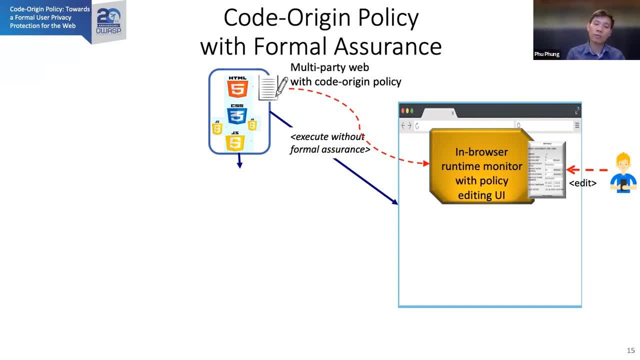 the monitor, but there's no, no formal insurance right. so my, my research now is try to ensure that when we have a code origin policy like this, we also have a tool to generate the formal like proof that we found a certificate right. so this certificate will be together with with the, the code and also the policy. 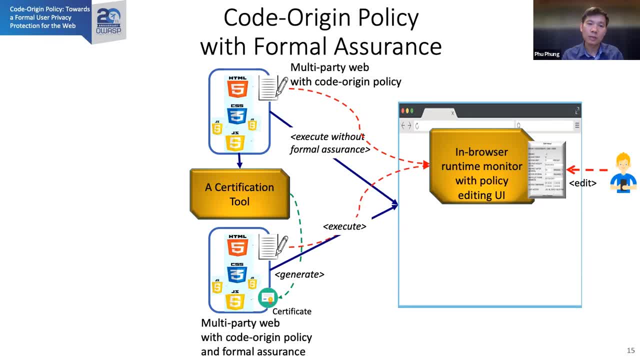 and at runtime it will be verified the if the code already had the code origin policy. so that is, granted, two things right. the first thing is it can be monitored to ensure it's not violated, violated policy. the second thing is that to ensure that this code have this kind of enforcement at runtime, and so so at for now, we explore a couple. 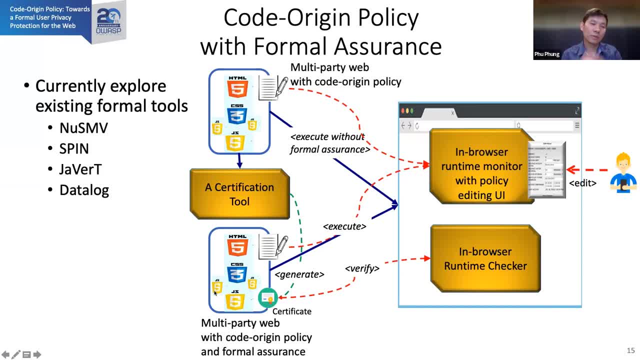 of tune and um, like, for example, the current tune in in informal methods, but um, we didn't have a like the final result that yet, but we are. we still working on like, okay, how we generate this uh uh policy and uh, i mean the certificate, and how we verify this. 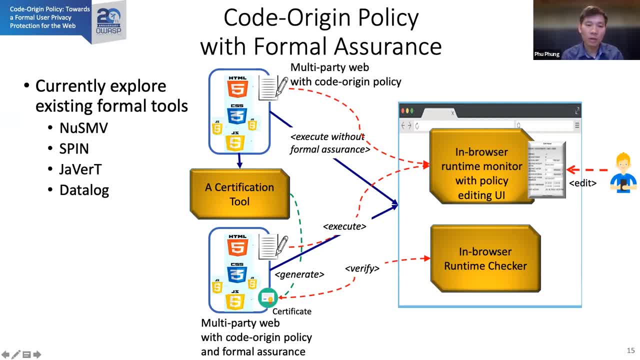 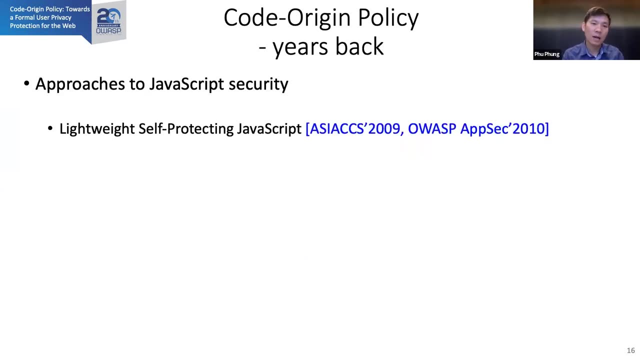 right so, um right. so in the team up, um like my research, i just want like um i we do for this uh anniversary, uh event, right. so i just review about uh the related work, my work that related to um call a integration: take those helpful skills, uh, they will be. 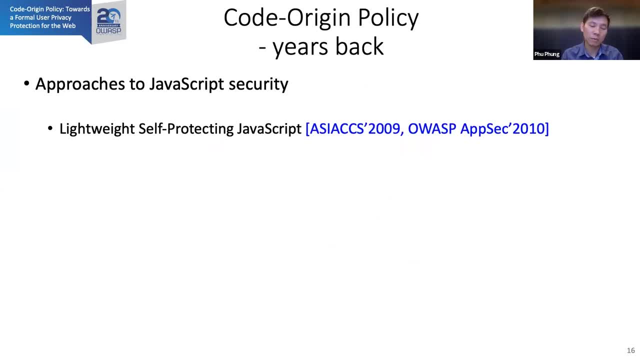 比 peripherals and date bursts. so i work with a lot of computers, andissa, and it just generally go in a pretty ohne Goal aspect. you know um. so ARS hon talki on how, Especially when, like at the end of the program t or gotOOS ming. 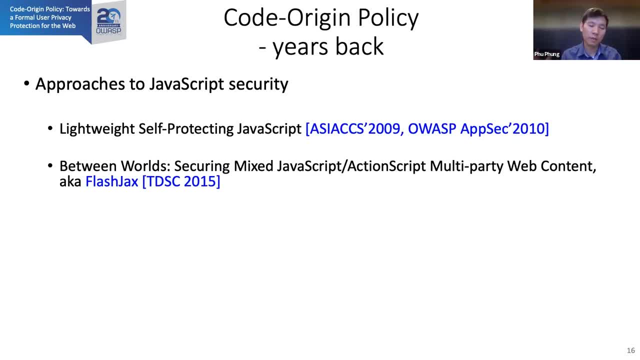 because it seems like, like i mean the, the things which we add, um, like the other uh things that we'm going to play around with, Like two things: policy for different origin, and recently i moved to the code origin policy that i just mentioned, and i also provide the mechanism for the user to modify the the policy at runtime as well, and 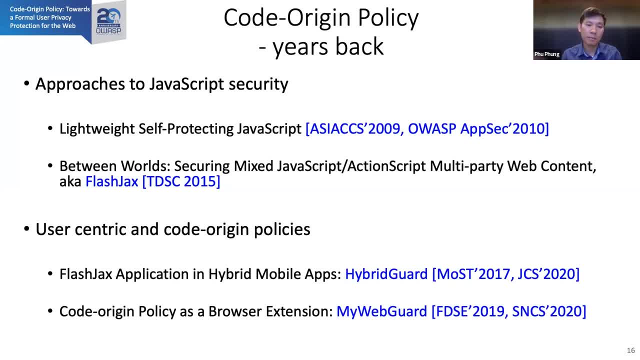 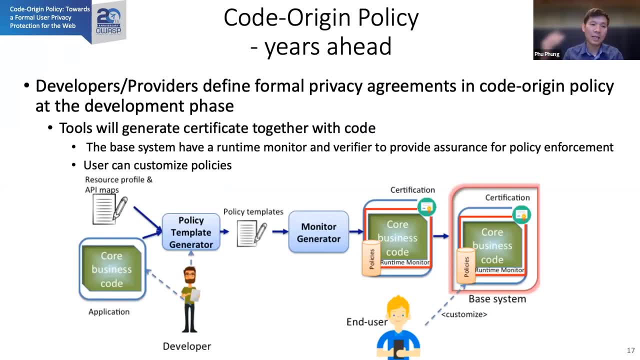 i just have a first prototype in code origin policy implement in the browser, so in in a long-term vision. um, i just mentioned to you the idea here is that, um, we can have like the code origin policy with kind of the formal privacy agreement is not just a test, but 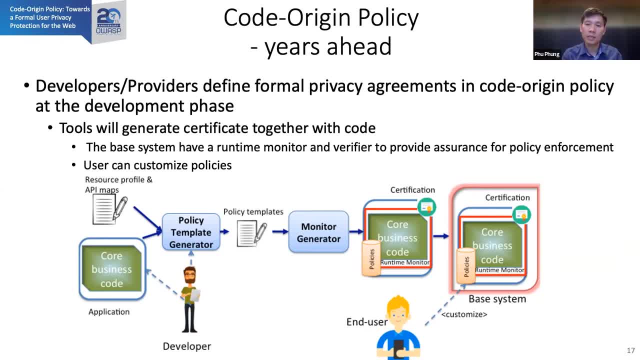 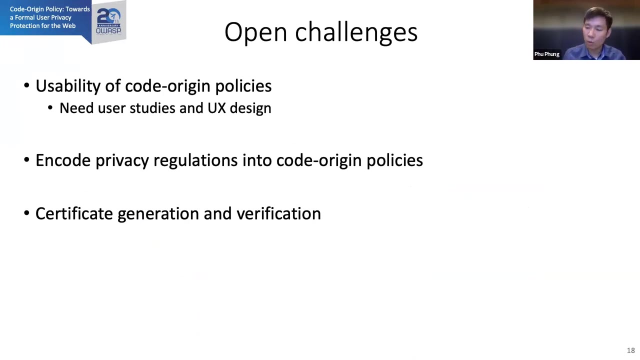 there are some formal way to define that in the code origin policy at the development phase and then we will use the tune. we develop a tune to ensure that the certificate will be chan generate and will be verified at the at the runtime right. so there's a lot of challenges here and, for example, what type?